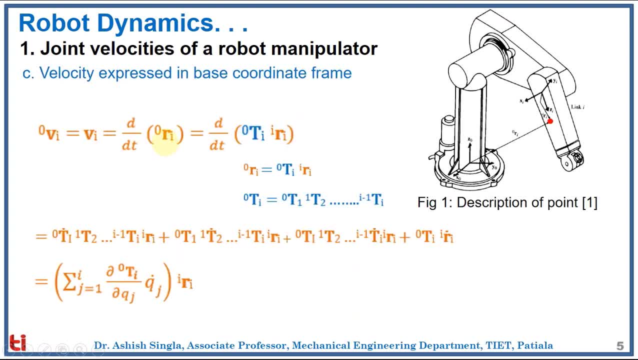 Now let's understand how is a transformation matrix done, point which is on link i is given by d, by dt of r with respect to base frame, equal to d by dt r with respect to ith frame, and this transformational matrix which converts that point to the base frame, and this transformation matrix is actually the multiplication of other. 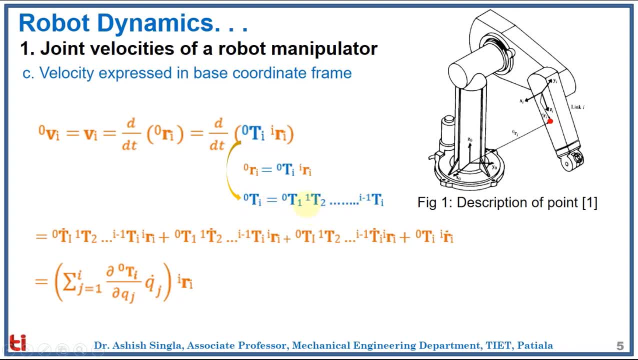 transformation matrices given here, and when we substitute this here and when we differentiate with respect to time, we get this expression and we find that the last term in this expression actually is zero, because we are differentiating point r, which is present in link i, with respect to ith frame, so that value is zero because that distance does not change. this is possible. 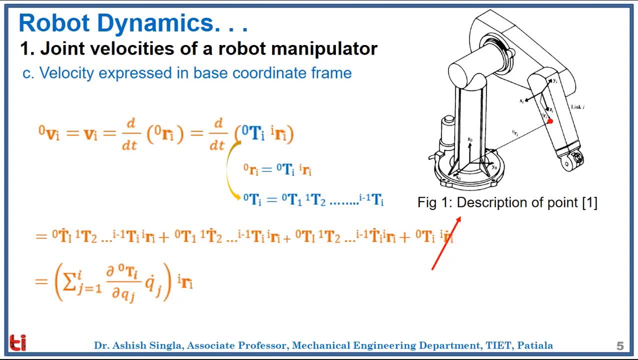 only for a rigid body, and in case of flexible bodies, this term is not zero. this whole expression can now be written in this form. now our area of interest is this circled term, which is partial derivative of the transformation matrix with respect to a generalized coordinate. it is a generalized coordinate because it 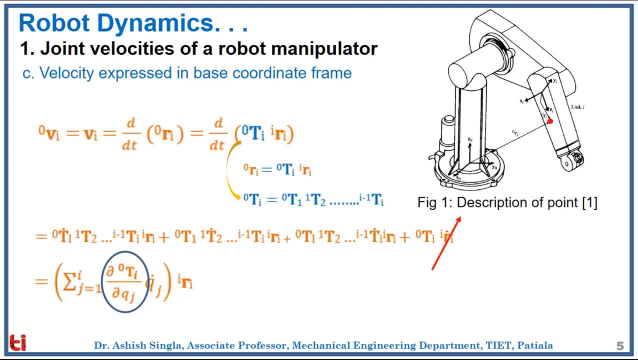 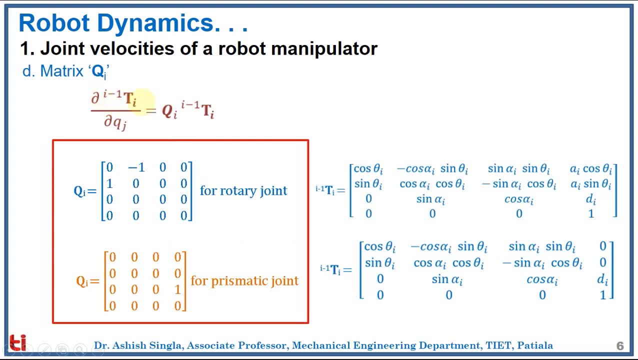 can be a revolute joint or a prismatic joint, so it can be an angle or it can be a displacement. now how do we find the partial derivative of this transformation matrix with respect to this generalized coordinate? so we grab on the hook that here is a the proportional Transformationaloras at sentimental. 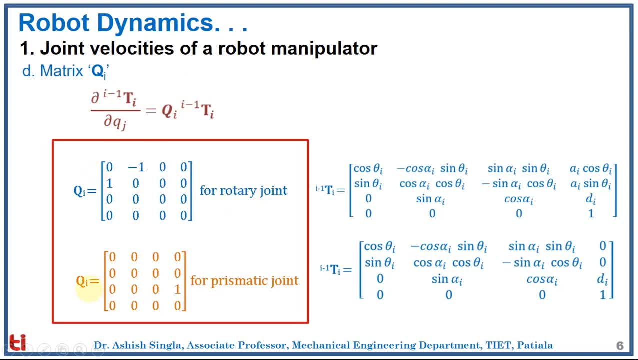 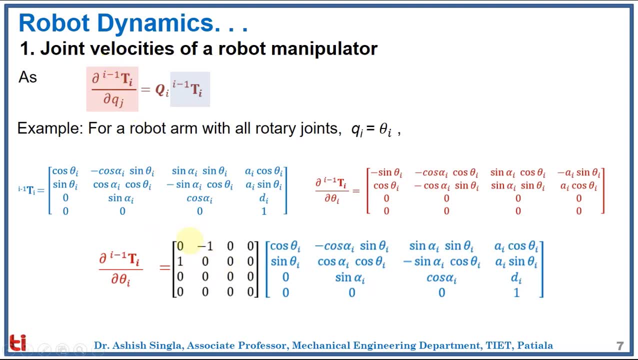 맞아요. this value is actually equal to this transformation matrix multiplied by another matrix, which is this matrix for rotary joint and this matrix for prismatic joint. now let us see. how did we get this value of this matrix? Mass13 왔? if we compare the transformation matrix for a rotary joint, that is Qi, is theta i. this is the transformation matrix and this is its partial derivative. If we compare the transformation matrixfor a rotary joint, thatis Qi, is θ I. thisis the Transformation matrixand. this is it's partial derivative. thoui. this is the personalized step too. 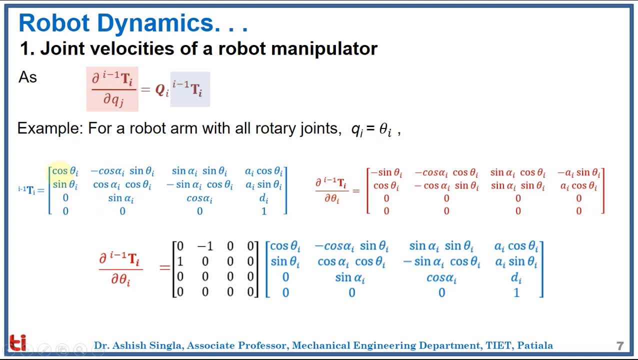 with respect to theta i, that is cos theta i. the derivative is: minus sine theta i. minus cos alpha i sine theta i. the derivative of this term with respect to theta i is: minus cos alpha i cos theta i. in this case, alpha is treated to be constant. now, when we compare these two matrices, we find that 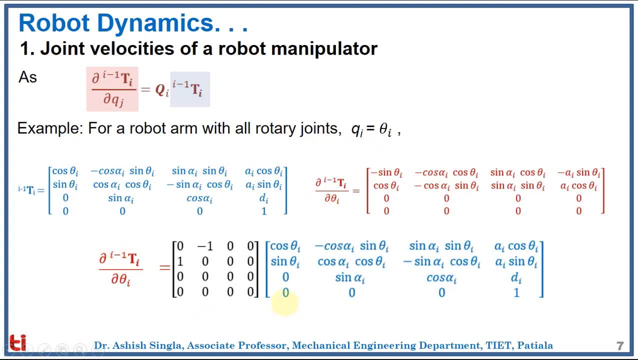 the second matrix is actually a multiplication of the first matrix with this term. for example, let us consider the first row of this matrix and the second row of this matrix. the terms, elements of this matrix, the elements of this row are same, and that is why we have a 1 here. 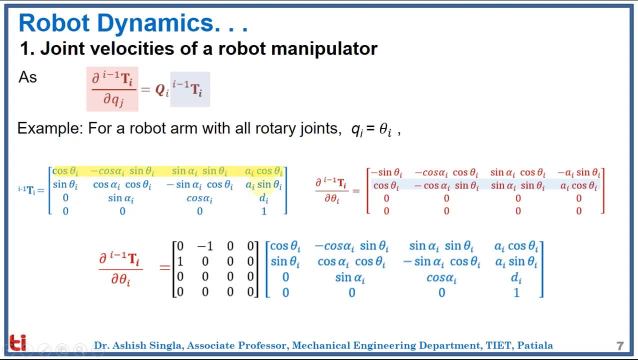 and if we see in the second case, the second row, this row is actually multiplied by minus 1, and then we get this row and this minus 1 in this matrix is because of that. so hence we get this Q matrices by comparing these two. this is the final. 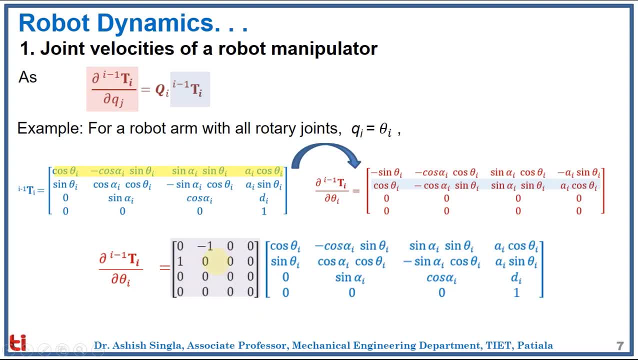 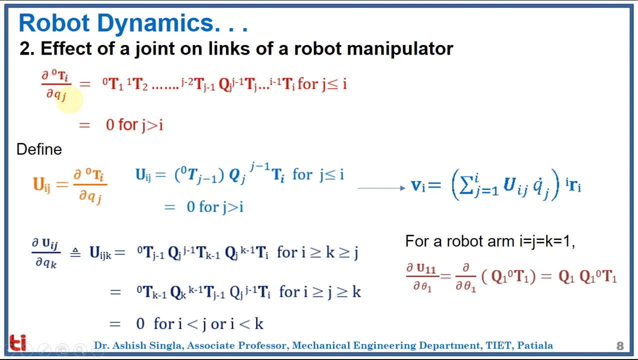 Q matrix, which is different for rotary joint and prismatic joint. now, this partial derivative of transformation matrix with respect to generalized coordinate can be expressed in this form: for J less than or equal to I, that is, number of joints are less than or equal to number of links, and is zero if the 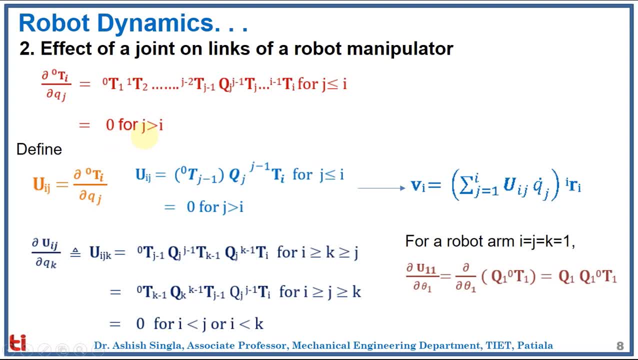 joints are more than links. if the joints are more than links, then that joint has no effect on the link, hence it is zero. now we define a new term, Uij, to actually represent partial derivative of the transformation matrix with respect to generalized coordinate, and Uij is this expression for J less than or equal. 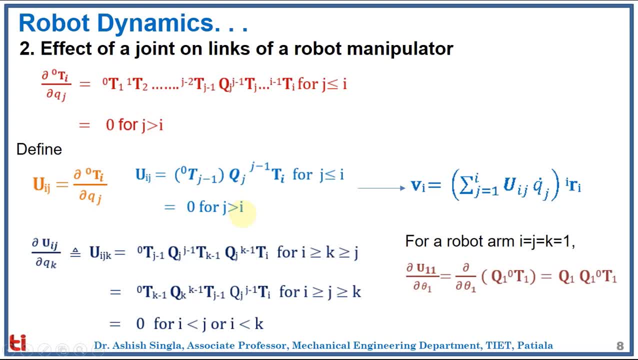 to I equal to 0 for J greater than I. we define another new term, Uijk, which is nothing but partial derivative of transformation matrix, and this is the partial derivative of the previous term with respect to Qk. that is, we are actually trying to get the interaction between two joints on a link in this. 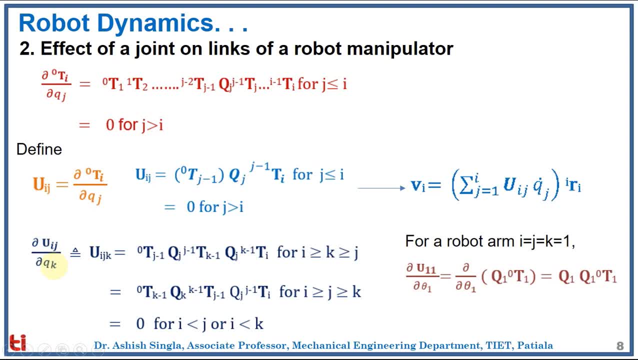 case, I is link, J is a joint and Q is a joint. so this expression, when we differentiate it with respect to Qk, we get this expression and while differentiating this expression, we can use the property that Qk is equal to. I, the partial derivative of transformation matrix, with respect to generalized 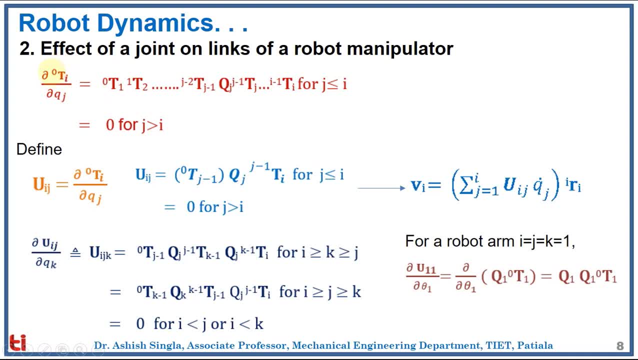 coordinate is actually Q times the transformation matrix. so we get two times Q here. let us consider an example for a robot arm, for a single arm, number of links I is one. number of joint is one and for comparison there is another joint. the total joint is actually one. this is considering the effect of other joint, which is one joint. 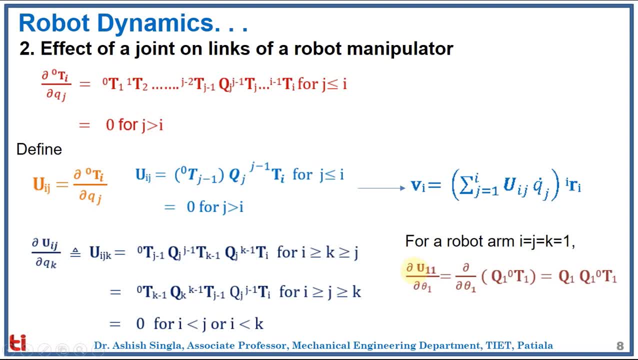 which is also one. there is no second joint. so partial derivative of U11 with respect to theta1 is nothing but this expression, and when we expand this we actually get Q1 dot, then partial derivative of this plus Q1, partial derivative of 0 or T1, the derivative of Q1. 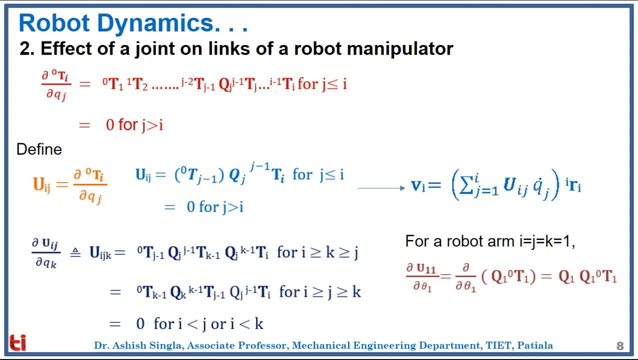 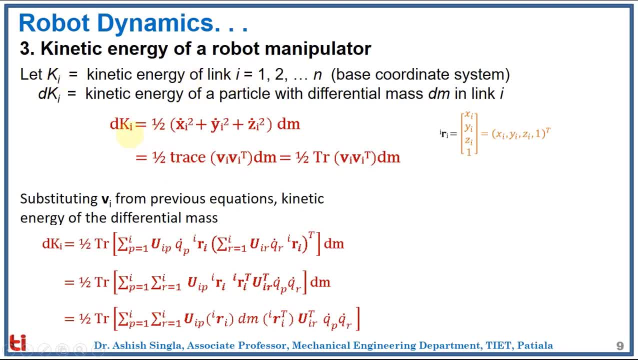 Let Ki be the kinetic energy of the link and D Ki is the kinetic energy of a particle with differential mass, dM in link I. then D Ki is given by this expression, which is nothing but half Franck's linear instead of Cj, and is nothing but half. 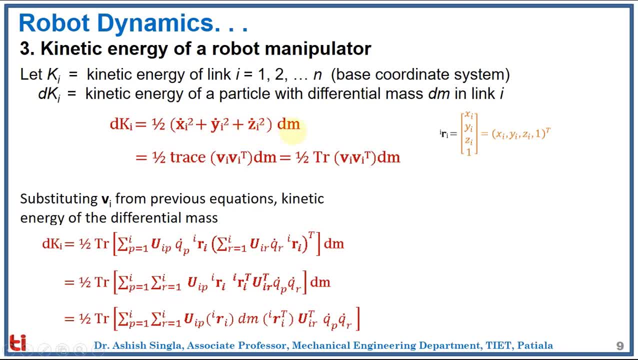 x i dot square plus yi dot square. Dm kinetic energy, we know, is half mv2 and v is nothing but square root of this expression. so v square is xi dot square plus yi dot square plus zi dot square. now how do we get these values? for example, we 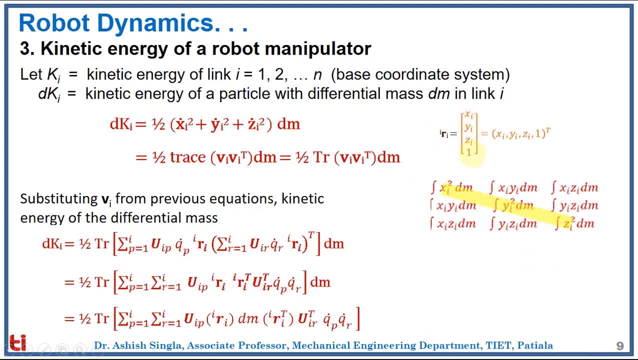 know that this point R can be defined by xi yi zi 1. so when we multiply by R again, we get a term similar to this matrix, where xi square, yi square, zi square are actually the elements of the diagonal. and now that we have these terms, the sum of these terms will actually satisfy here. so this is: 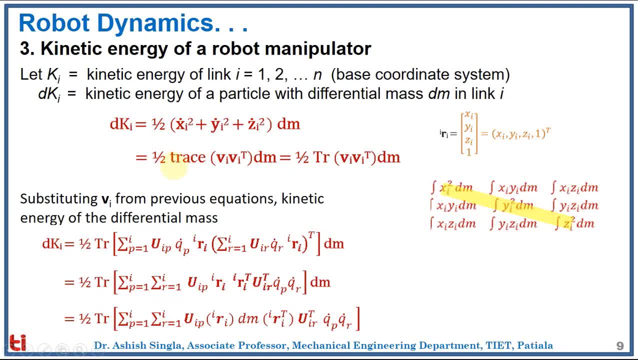 nothing but the sum of the diagonal elements is nothing but the trace of the matrix, which is equal to half trace vi, vi transpose dm. if this is R, we will be xi, dot yi, dot zi, dot 1- sorry, here it is 0. and when we multiply, 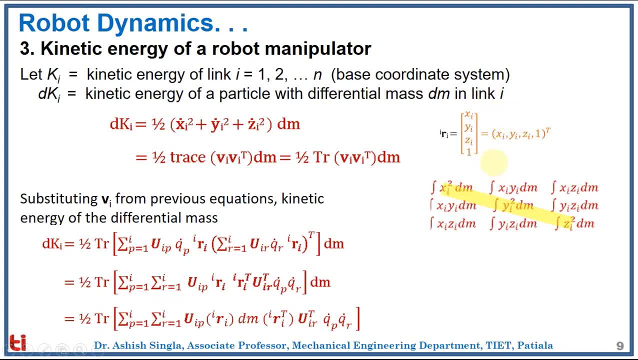 by xi dot yi, dot zi, dot 1- sorry, here it is 0- and when we multiply by R, we get a again. with xi yi zi, we actually get this matrix, and the sum of diagonal elements will actually give us the value of this term, which is nothing but trace. 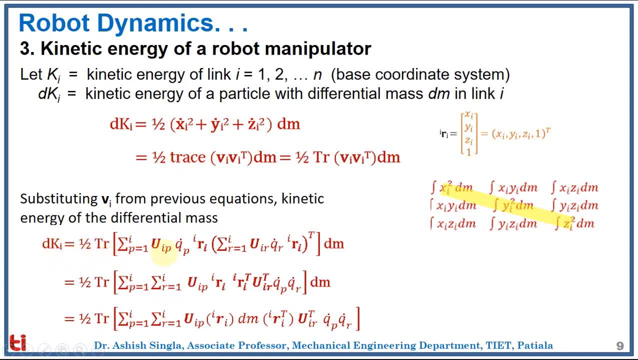 now, this kinetic energy can now be rearranged in this form. this term is vi and this term is vi transpose. it can be rearranged to this form. and now the same thing can be rearranged finally into this. here we find a term, R MR, which is nothing but MR square. MR square is nothing but moment of inertia. 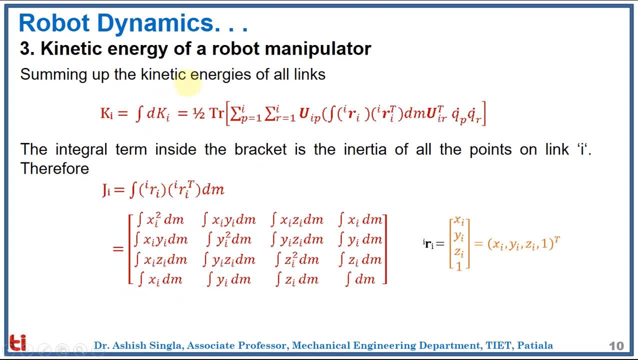 so summing up of kinetic energies, of all links, is nothing but integral dki equal to half trace of this expression. and in this expression we find that this value, which is nothing but R, R, transpose dm, is actually given by inertia tensor, and inertia tensor is a matrix which actually gives the idea of moment of inertia of the 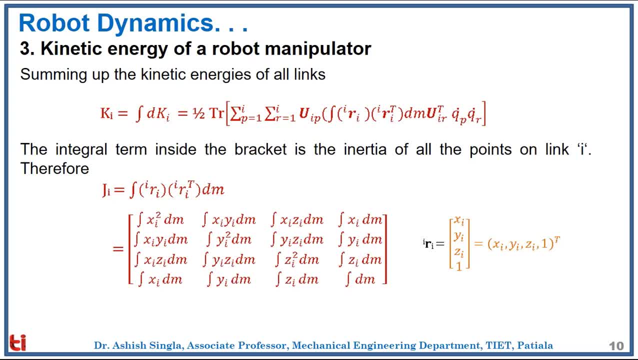 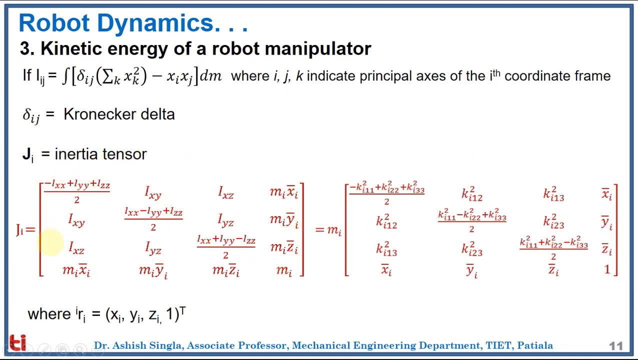 3d object when it is rotating with respect to different axis, and this inertia tensor can also be expressed in this form, where ixx, iyy, izz are the moment of inertia about the principal axis, and this inertia tensor can also be expressed in this form: 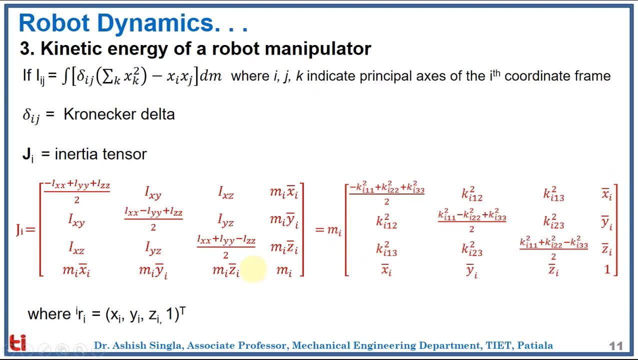 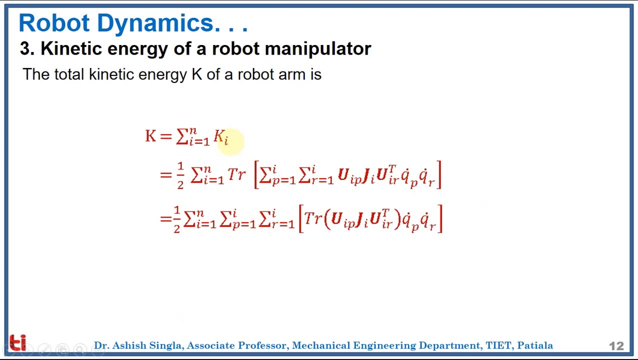 where k is the radius of gyration. this inertia tensor is different for different bodies and based on the type of manipulator link we can find out this inertia tensor matrix. the total kinetic energy is nothing but sum of individual kinetic energies of every link, and this is the final expression which we get now. 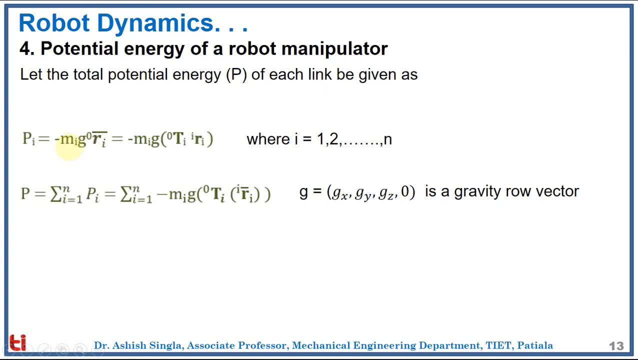 the potential energy of each link is given by mg into this distance from the zero base position or the relative position, so which is nothing but MIG, into R. and this R with respect to base frame can be written as R with respect to ith frame of link I multiplied by this transformation matrix. this is for a single link and potential. 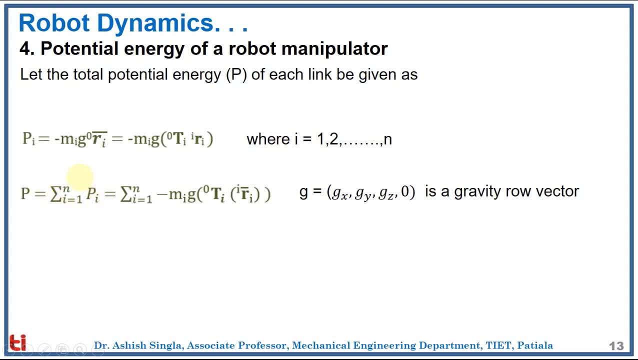 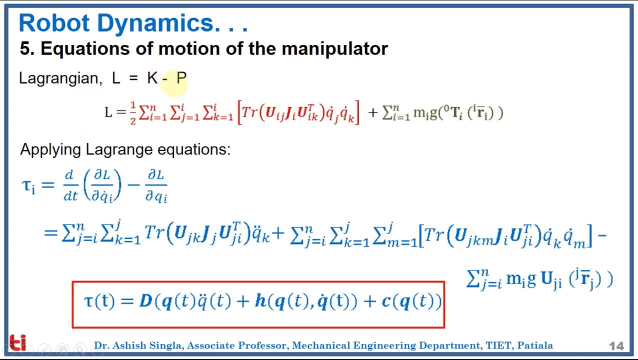 energy of all links is equal to the sum of individual potential energies, which is nothing but this expression. Lagrange energy is nothing but the sum of individual potential energies, which is nothing but this expression. Lagrangian is nothing but total kinetic energy minus total potential energy, which, from previous equations, if we substitute it here, we get this equation. 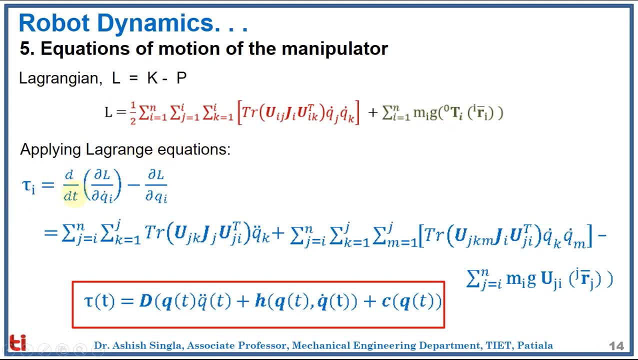 now applying Lagrange equations, that is: tau i equal to d by dt partial derivative of Lagrangian by qi, dot minus partial derivative of Lagrangian with respect to qi. we get this expression. when we substitute L here, partial differentiate, we get this and this term. 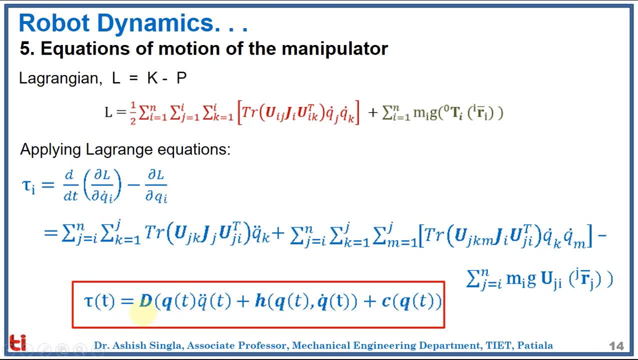 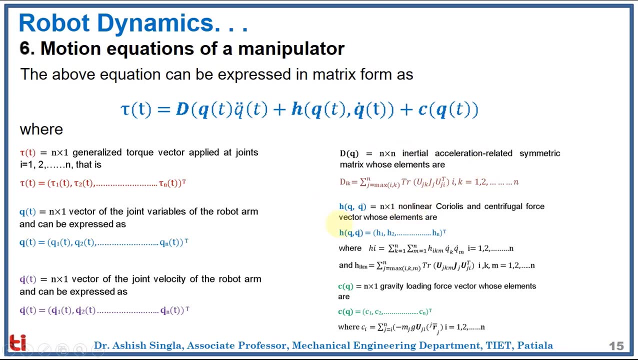 can be grouped as this equation: where B represents the inertial terms, which represents the core, less and centrifugal terms, and C represents the gravity terms, the same thing is expressed here in detail: where D represents the inertial term, Sung represents the Coriolis and centrifugal. 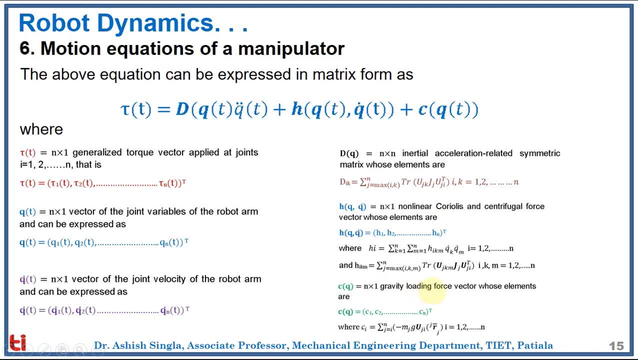 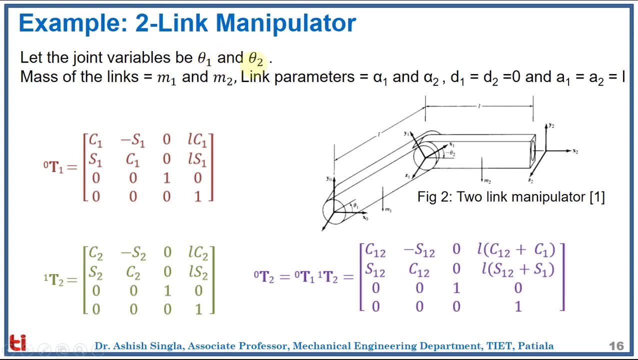 force vector and C is the gravity load force vector. let us consider the example of a to link manipulator. the joint variables are theta 1, and doesn't matter, and theta 2, that is revolute joints. mass of the links m1 and m2, and the length of each link is l. 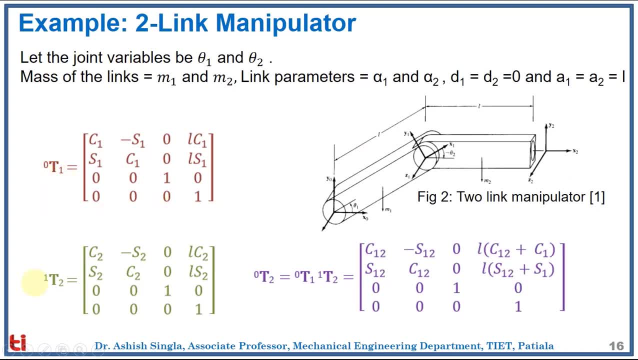 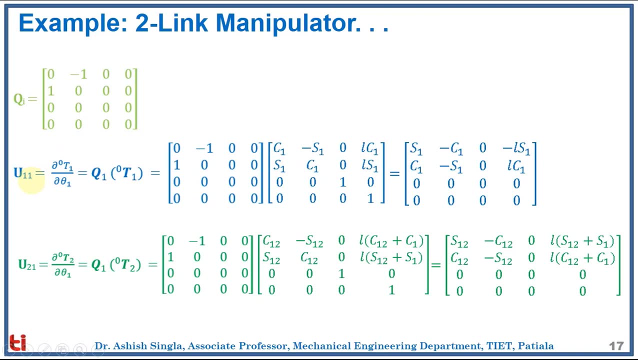 this is the transformation matrix for first frame with respect to base frame, second frame with respect to first frame and this is a transformation matrix for second frame with respect to base frame q. in this case is this matrix because it is revolute. joint u11 is given by this expression. 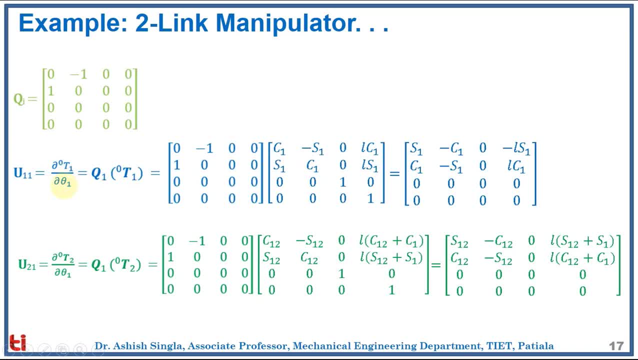 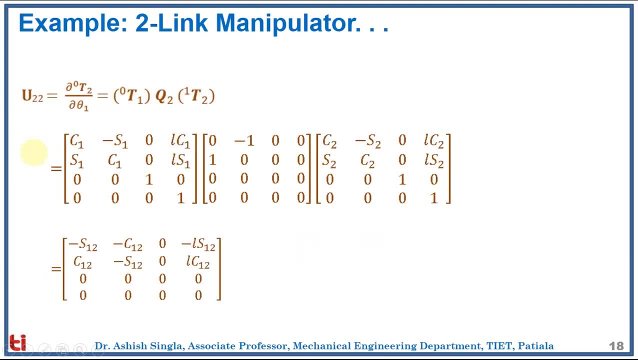 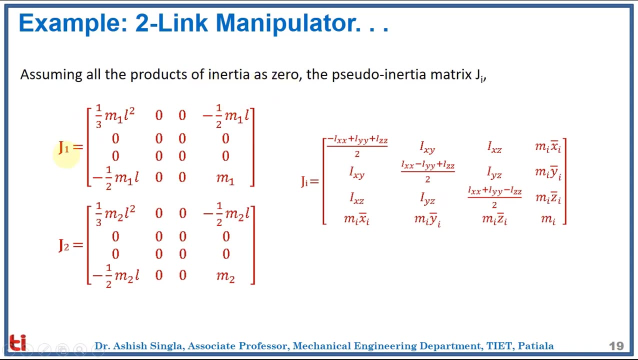 which is nothing but partial derivative of transformation matrix with respect to theta 1, and it is given by this matrix. similarly, we find u21 and u22, assuming all the products of inertia as 0. the inertia tensor for first link is this and the inertia tensor for the second link is this matrix, and this matrix is for a link which. 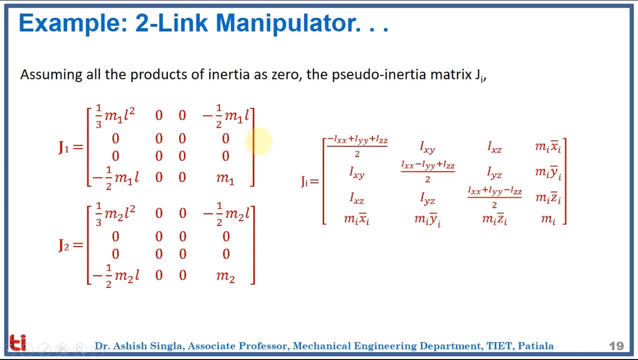 is assumed to be iscrchain slender. Slender means the length is more than the other two dimensions, That is, the other two dimensions are very small when compared to length. For this one can refer the inertia tensor of a rectangular link or a rectangular object. 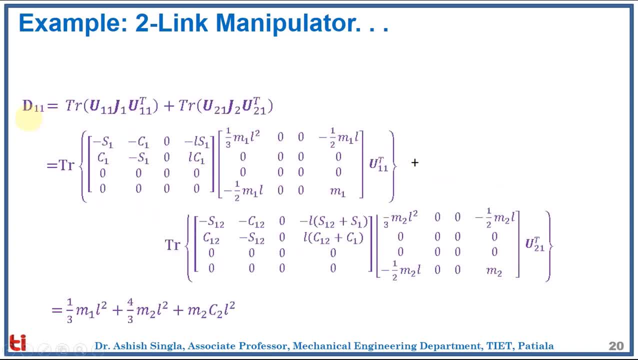 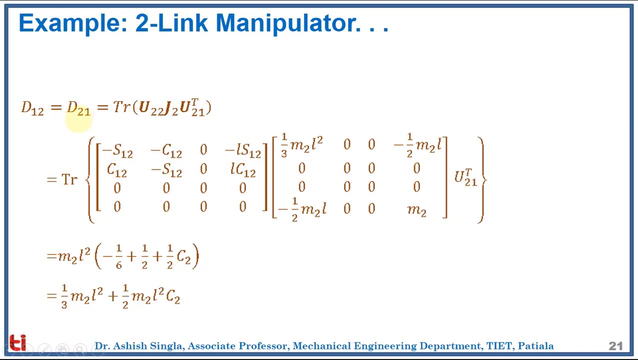 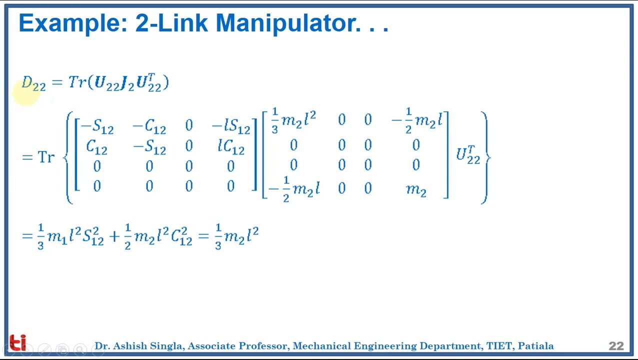 for this matrix. Now we find D11, which is given by this expression, That is, we multiply these matrices and then find the trace. Trace is nothing but the sum of diagonal elements. Similarly we find D12 and D21, and similarly we find D22.. All these terms D are nothing but the initial terms. Now we find the. 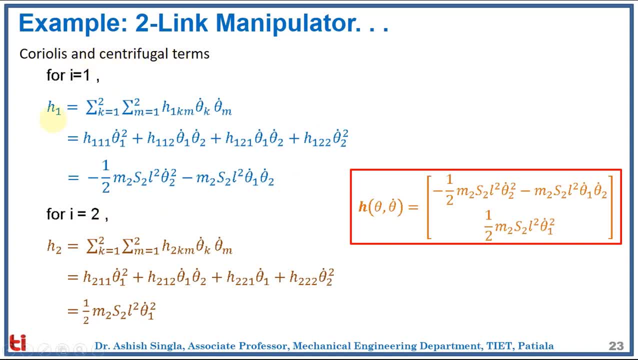 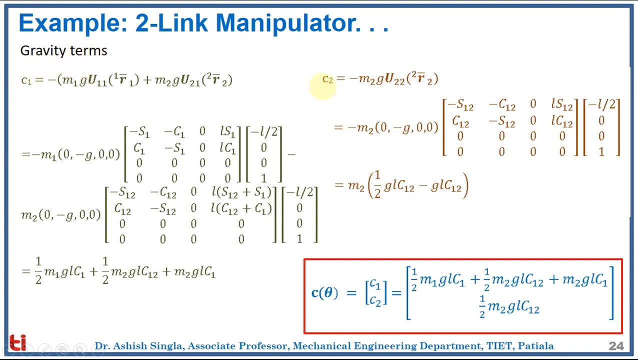 Coriolis and centrifugal terms- We have discussed this in the previous slide- and substituting 1 and 2 in the generalized equation, we get H1 and H2 and this is the H matrix. Similarly, C1 is a gravity term and also C2.. C1 is obtained by substituting 1 in. 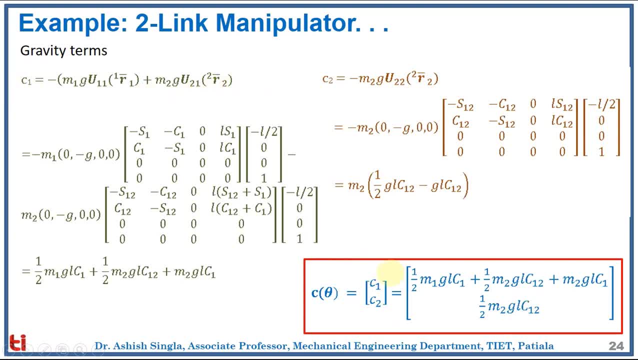 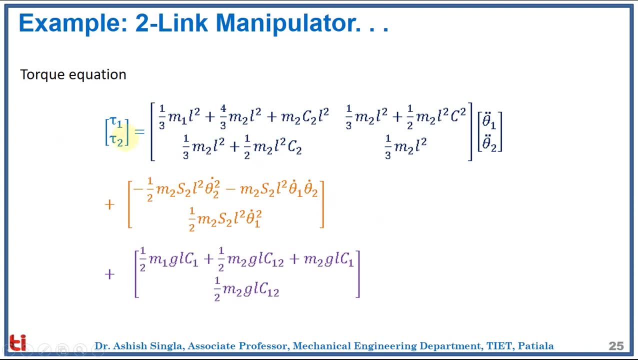 the generalized equation discussed earlier. This is the final matrix for gravity terms. Combining all these, we get the final torque equation, which is nothing but the inertia matrix. This is the Coriolis and centrifugal matrix and this is the gravity matrix. Let us discuss the generalized code for inverse. 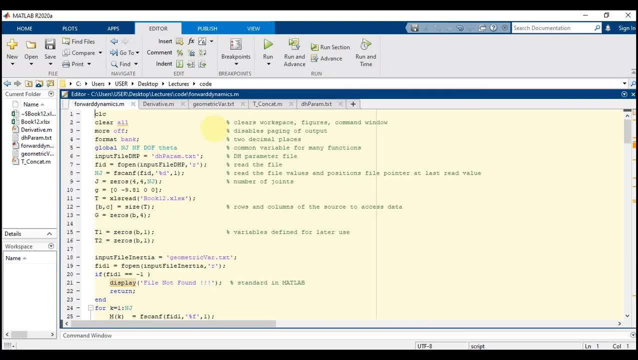 dynamics of the manipulator: Clear, all Clears, workspace figures command window Format which is of bank type, that is, two decimal places. Global variables: nj, nf, dof, theta. Global variables because these variables are called for many functions. We are reading the file dhparamtxt, which actually has the 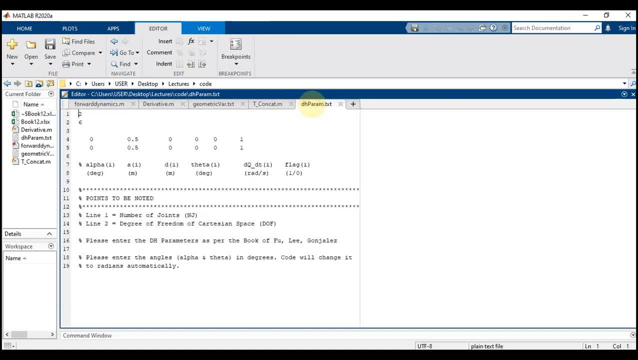 dh parameters of the tooling. So this is the dh parameter: alpha a, d, theta, dq by d, t and flag. This flag is 1 for revolute joint and it is 0 for prismatic joint, Though we have given theta and dq by dt to be zeros, here we have actually 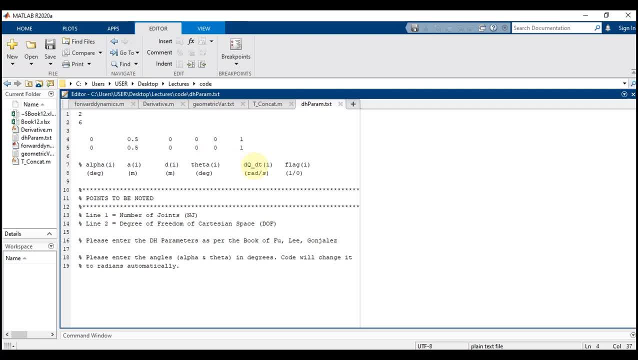 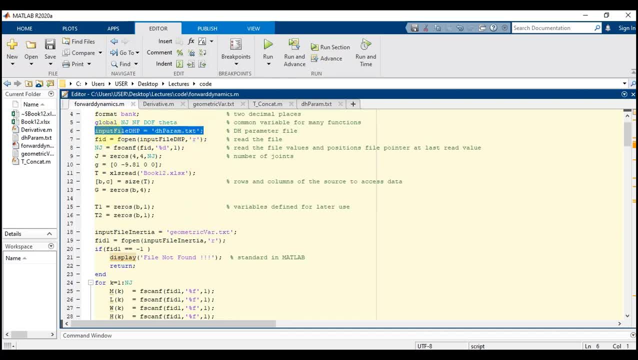 considered those values, which is discussed in the program later. After reading this dh parameter file: we perform this operation fscanf. fscanf actually reads the file dhparamtxt. We perform this operation. fscanf. fscanf actually reads the file values and positions. file pointer: at last read value, That is say for. 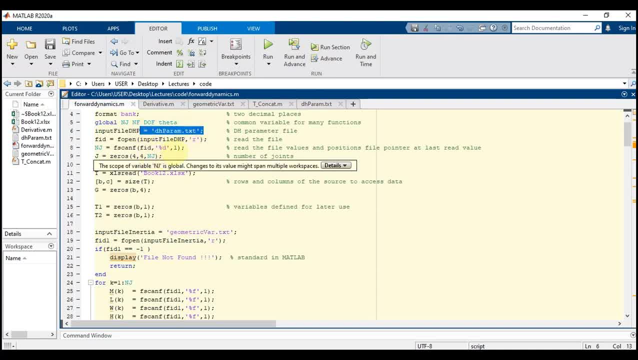 example, we are reading this text file. It reads the value present in the first row and next time, when we call this function again, it reads the value in the second row. This is the gravity matrix. Gravity is in negative y direction. XLS read actually opens the excel sheet, which is our source file here. Let us see. 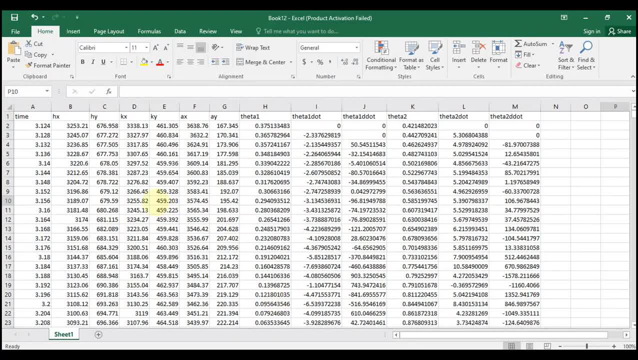 what is there in this source file? Here we have the time values, We have the coordinates for the starting of first link, ending of first link or the starting of second link and the ending of second link. From these coordinates we get theta1 and theta2 and from theta1 and time we can get: 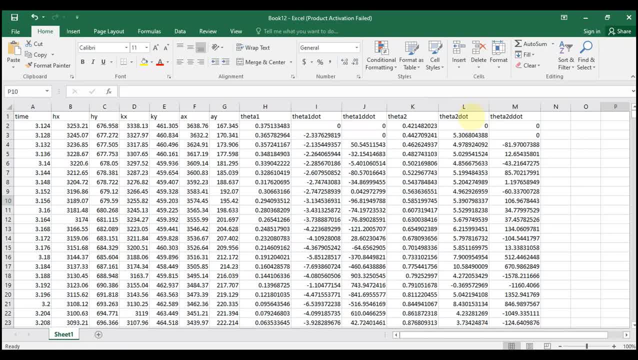 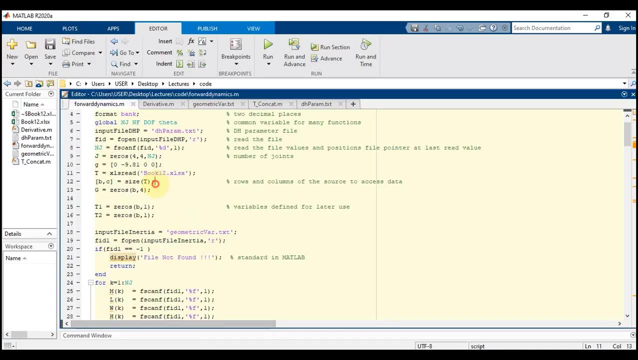 theta1. and theta2. using a matlab code and we can get theta1 double dot and theta2 double dot. Sometimes these values, theta1 and theta2, are directly given to us. In that case we don't require these coordinates. Now, BC gives the rows and 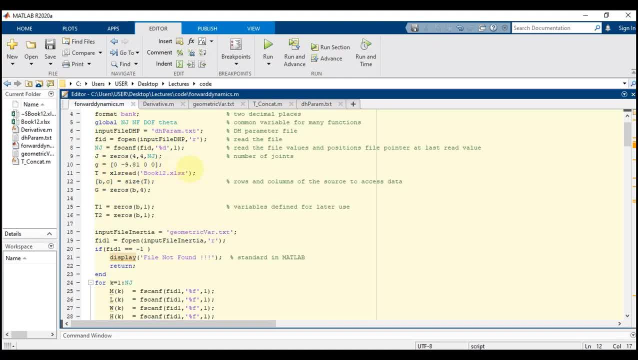 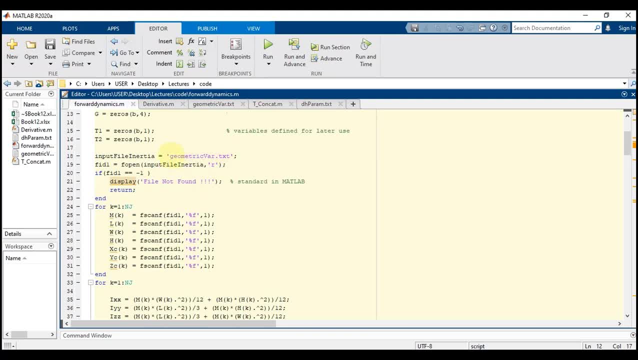 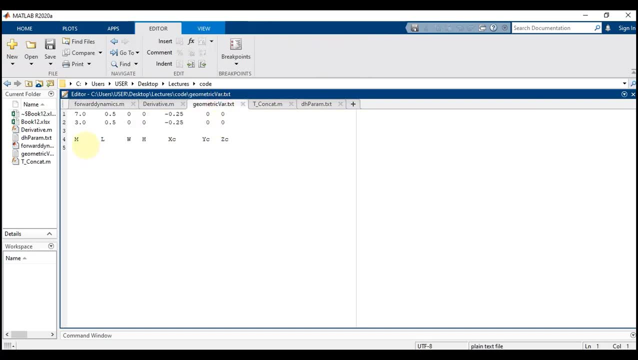 columns- value of this matrix or of this excel sheet which is read. We are inputting or reading another text file which has a geometric properties of the link, that is geometric vartxt. Here we have given the mass of the two links, say they are seven units and three units. 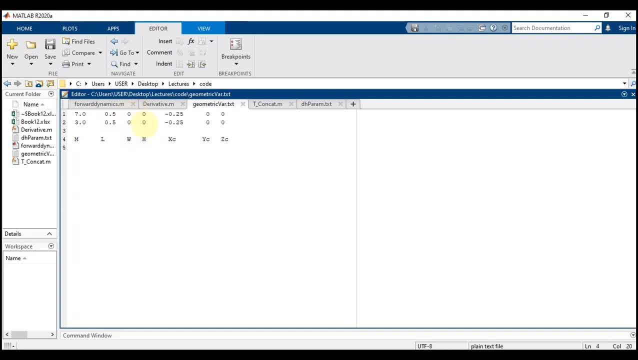 length, width and height, both are zero. for slender link, Xc minus 0.25 and minus 0.25. this is negative because for every link its frame is fixed at the end of the link. so when we want to know the center of gravity, because the frame is. 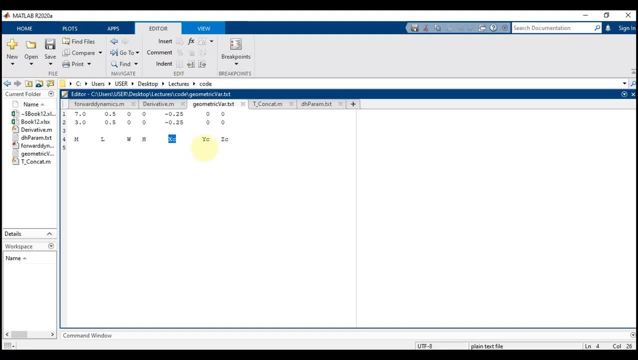 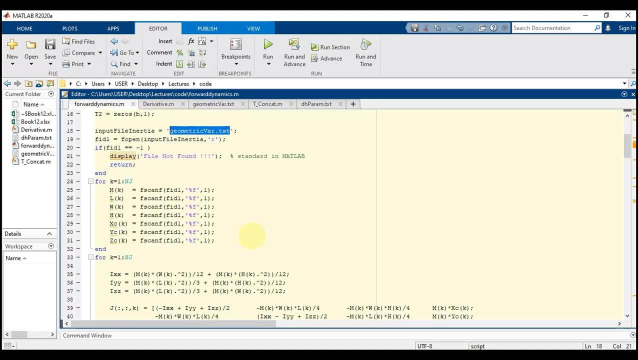 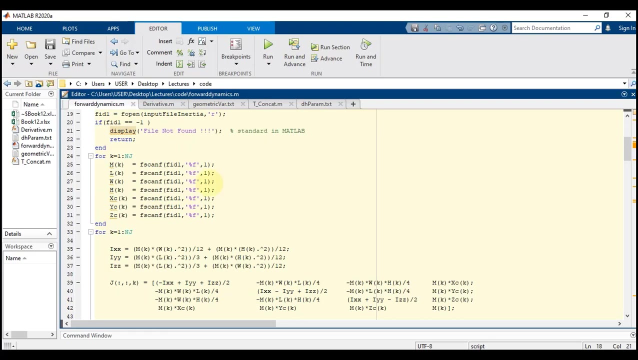 fixed. at the end of the link you have to come minus 0.25 units in the negative direction because the length of that link is 0.5 units and this is the same for both the links. FID is minus 1. it says: file not found is the standard used in MATLAB and this: 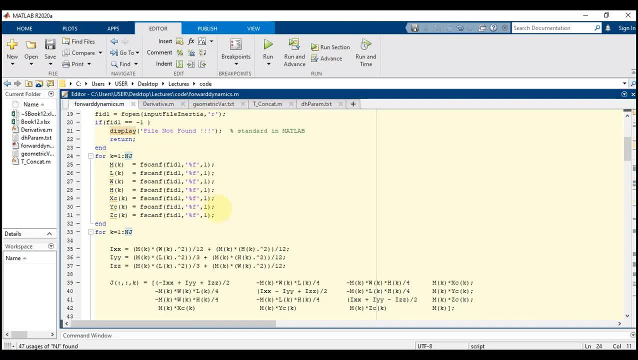 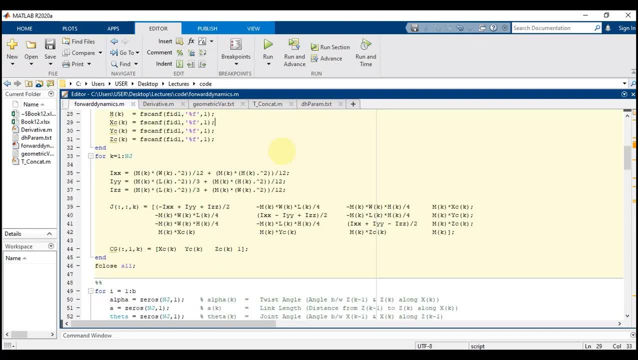 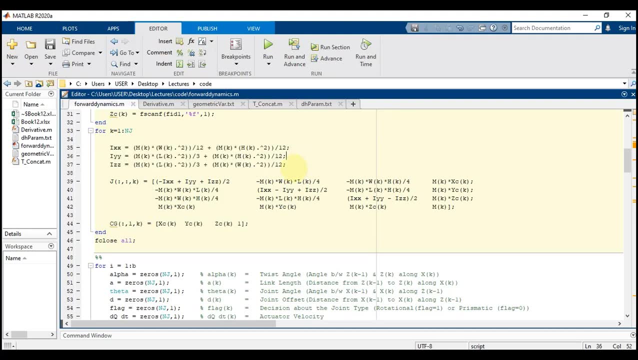 number of joints for the first link and the second link. for the end of link you have to come minus 0.25 because the the second link we actually read these values: mass, length, width, height and center of gravity. this is the moment of inertia of the link which we have. 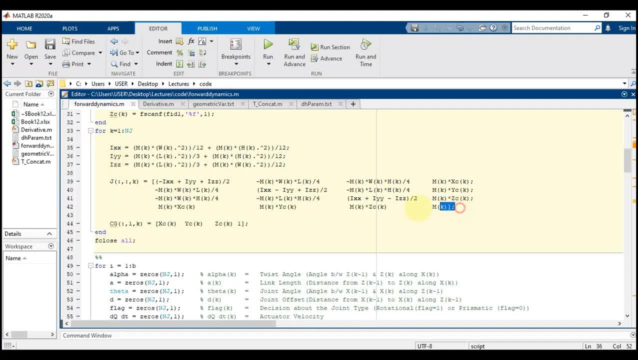 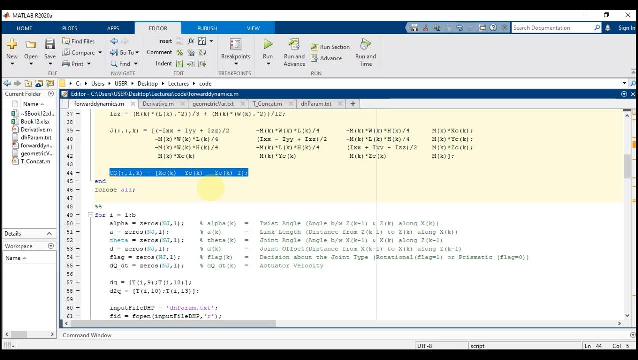 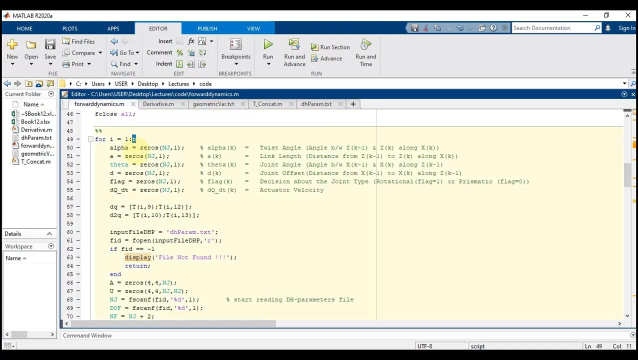 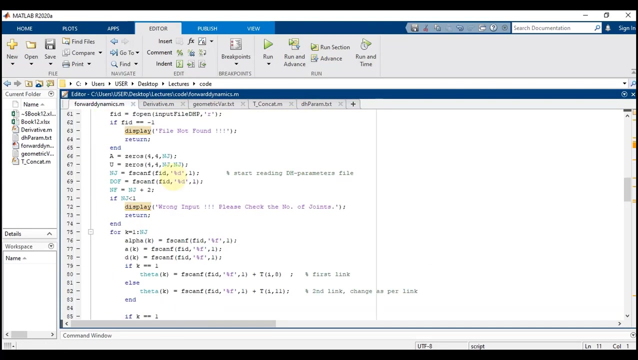 considered about the principal axis. this is the generalized inertia tensor. this matrix changes if the link is cylinder or of any other shape. the coordinates of center of gravity now for I, equal to 1 to B. we know that is the number of rows of that source file which we are referring. 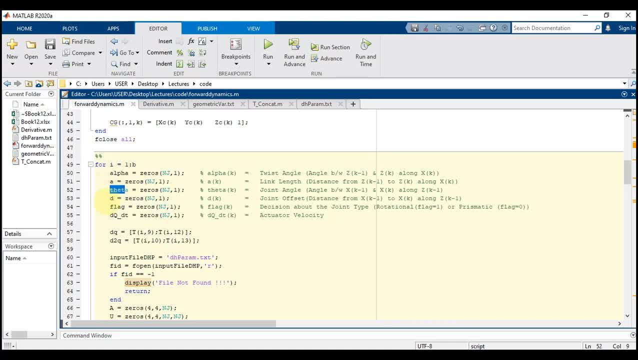 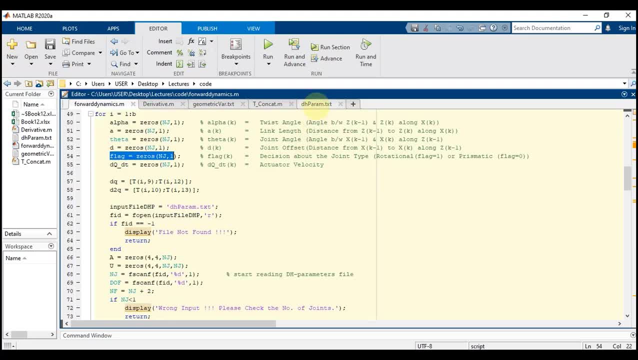 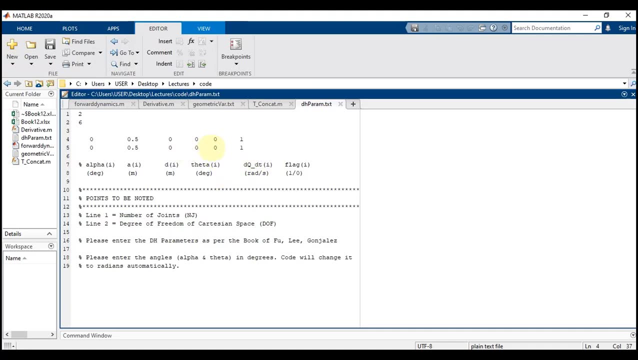 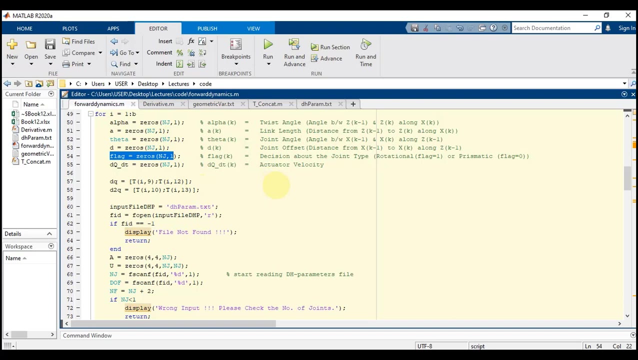 alpha A, alpha B, theta d and flag. we get from this file dh parameter file. so in this dh parameter file, as discussed earlier, theta and dq by dt are given as zero. however, those two values are actually inputted to get the torque values. dq is velocity, d2q is acceleration. 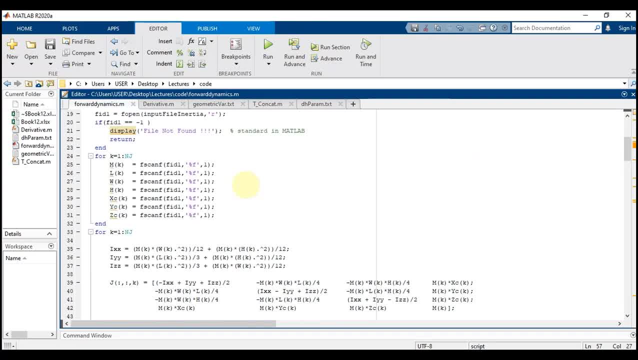 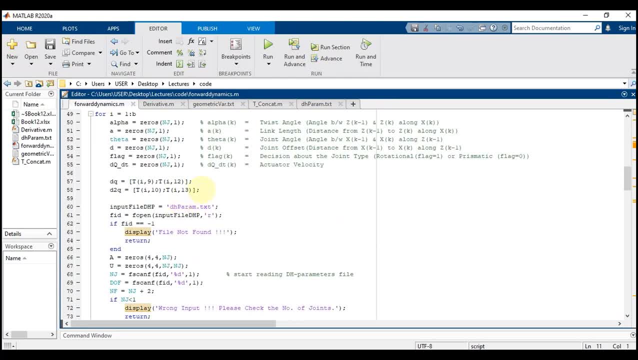 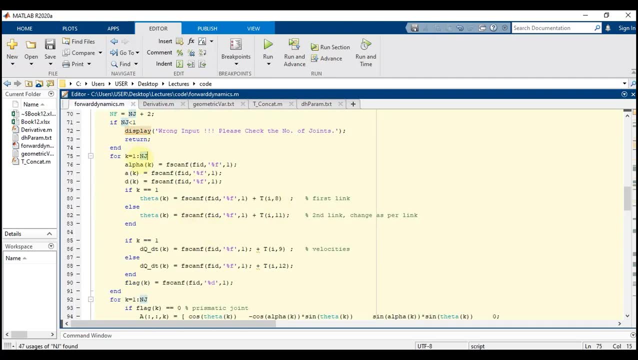 and this actually referring to the excel sheet which we are reading and the values are taken from that excel sheet. alpha is read from the file. a is read. d of k is read. for the first link, that is, if k equal to 1, theta 1 is nothing but this value plus ti of 8. 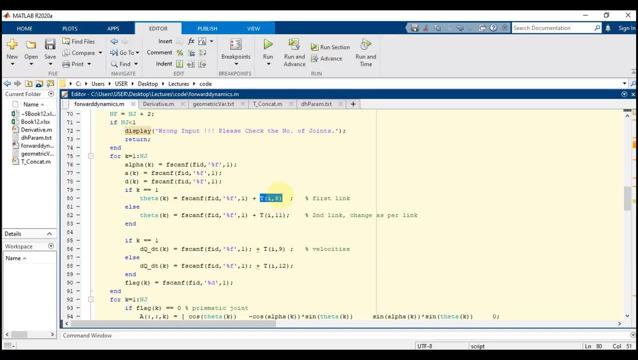 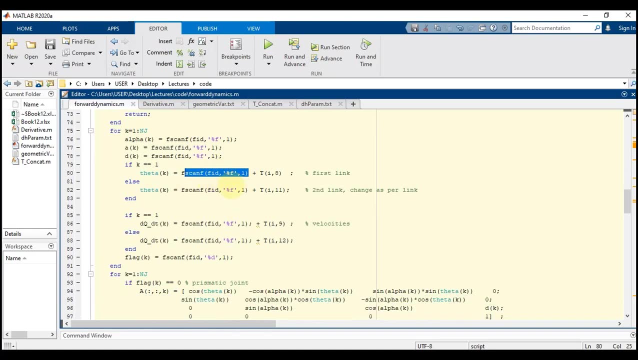 ti of 8 is the value present in the 8th column. if it is linked to, then we are referring to the 11th column. these two values are actually zero. because we have not mentioned any value here. we are taking these values from the excel sheet. a is read for absolute and absolute values. we are not mentioning any value here. we are taking these values from the excel sheet. 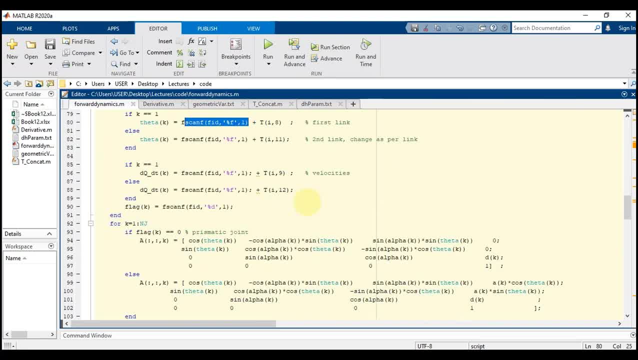 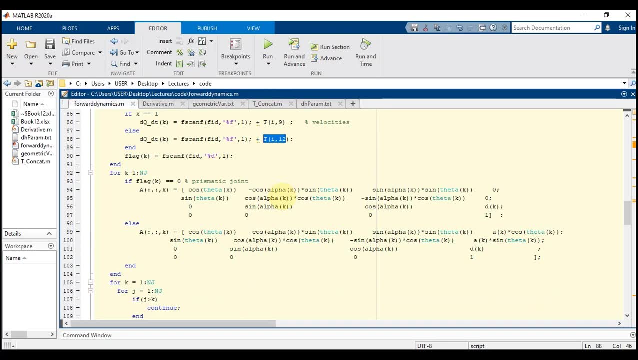 sheet and if k equal to 1 dq by dt, that is, velocity, is taken from the ninth column and k equal to 2, that is if it is the second link, is taken from the 12th column. if there are other links, like say three links, then k equal to 1, else if k 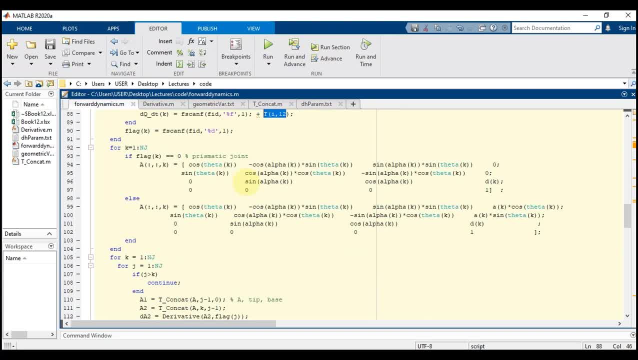 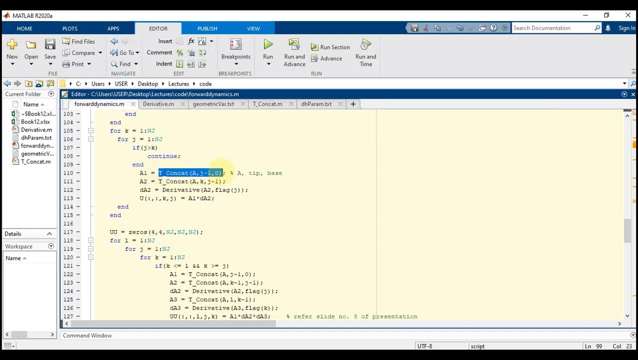 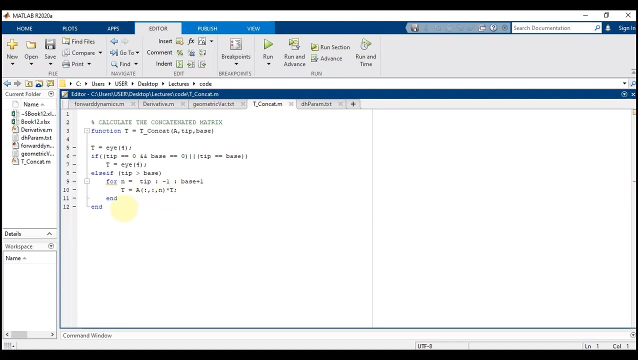 equal to 2, else. the third link is the transformation matrix for prismatic joint, transformation matrix for revolute joint. this t concatenate function actually concatenates the matrices. if you want to find the end frame with respect to the base frame, we actually have to multiply many matrices and this. 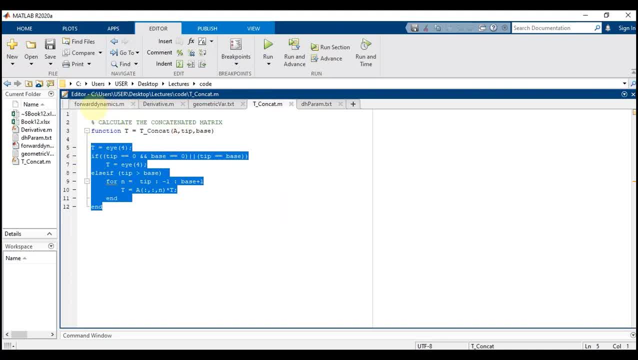 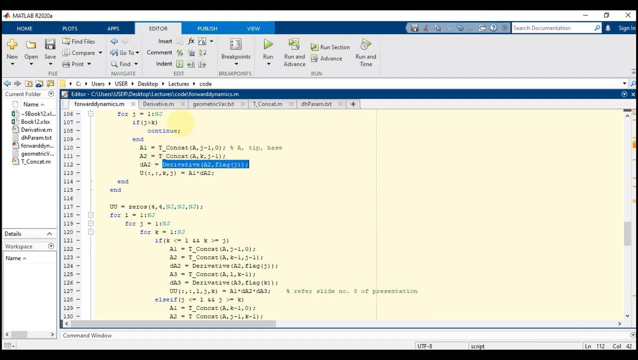 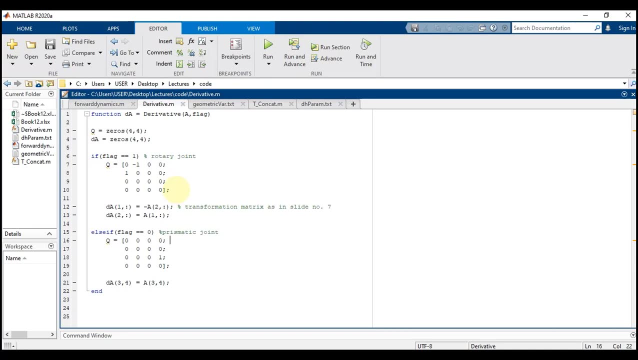 function does it and da 2 is derivative. a 2 flag J. let us see what is there in this derivative function. so, as discussed earlier, if we want to find the derivative of a transformation matrix, we actually have to multiply by Q. and this is the matrix if it is rotary joint. this is the matrix if it is prismatic joint. 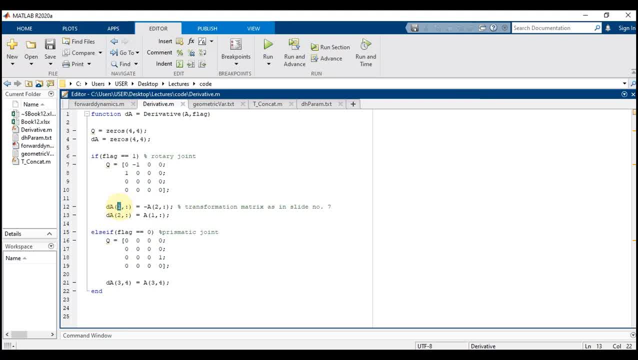 this term actually means that the first row of da is minus times the second row of a matrix and the second row of da is equal to first row of a matrix. so that can be verified by seeing these matrices, matrix rows and columns, if it is prismatic. 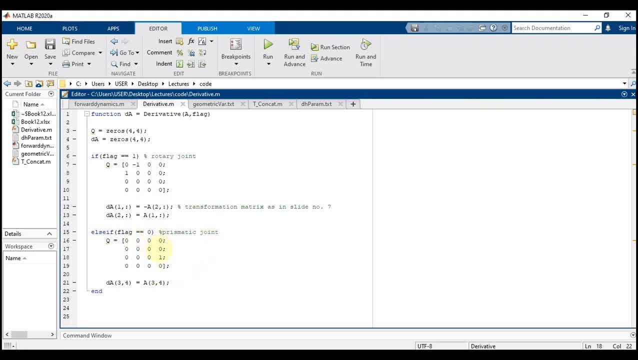 joint. we find that in third row and fourth column there is one one present, because for a prismatic joint only this matters and the angles do not matter, because it remains constant. the differential is zero. third row, fourth column of da matrix is actually equal to third row, fourth column of the a matrix. 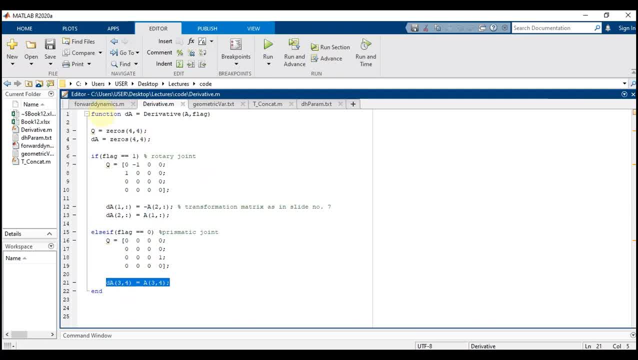 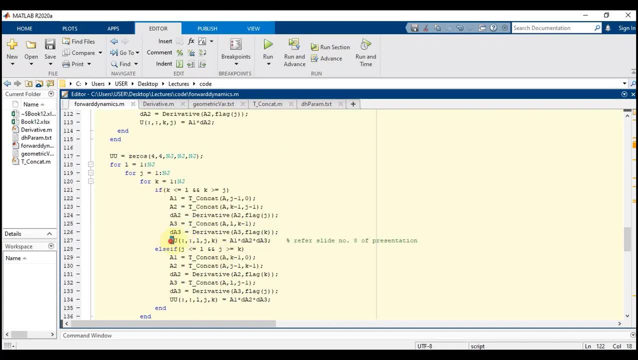 so this term represents that once the matrices are concatenated, then we find UU. that is which we have discussed in slide number eight of the presentation, which actually refers to the effect of joints on the links. da2 refers to effect of joint on a link and UU actually is the interaction forces between two joints or the effect of. 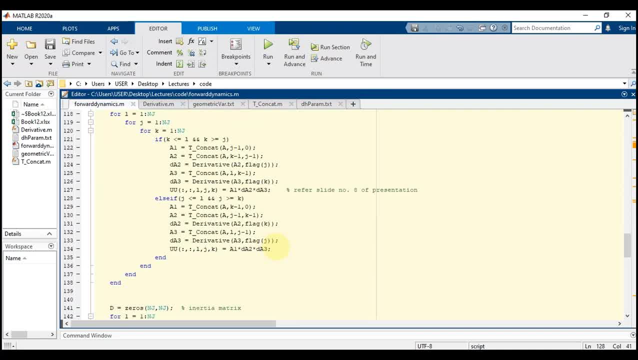 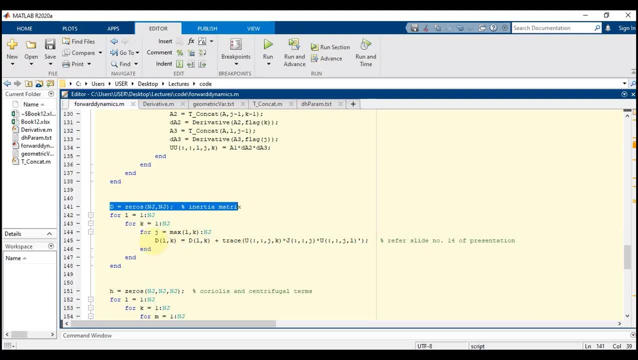 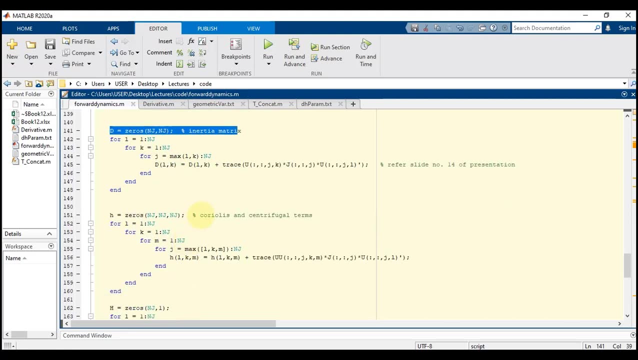 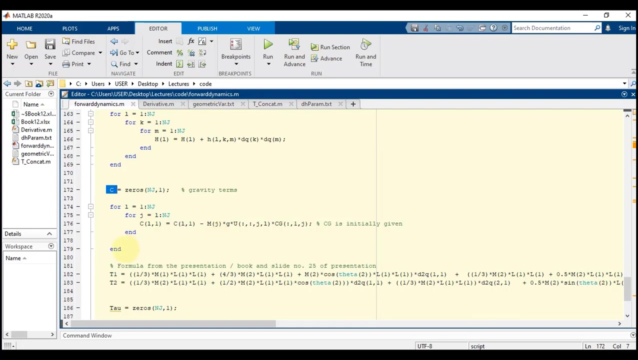 joints on a single link. d is the inertia matrix, which is obtained from the expression discussed in slide number 14 of presentation, the Coriolis and centrifugal terms, which is represented by H, the gravity terms, represented by C. so till here, this complete code is actually the general. 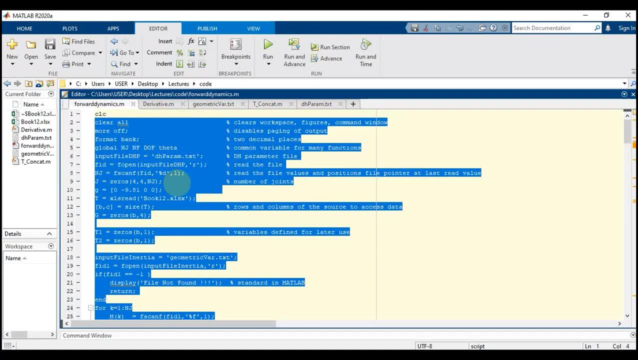 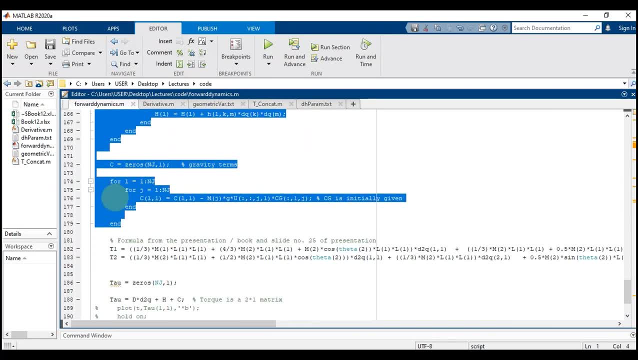 definition of the code. so till here, this complete code is actually the general definition of the code. so till here, this complete code is actually the general generalized code for inverse dynamics of a manipulator, and this is using Euler Lagrange method. to validate this code, which is highlighted in blue, we have also written: 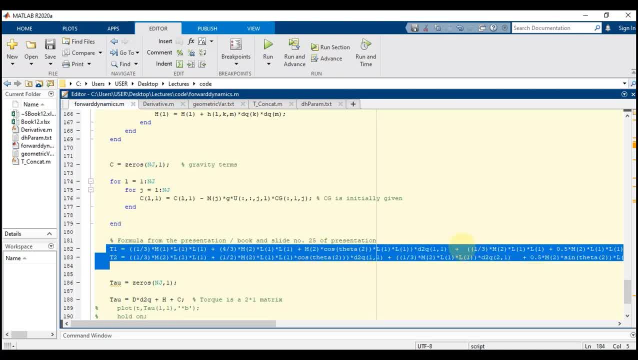 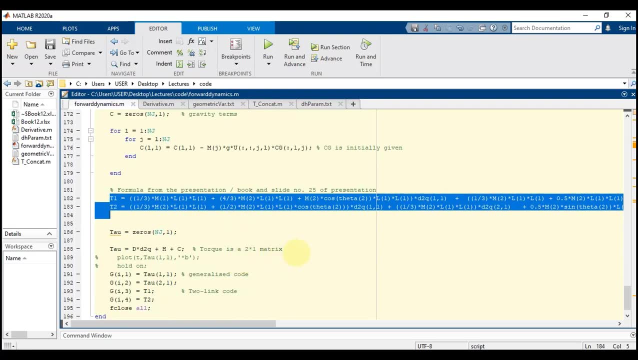 this expression which we got directly from the or ato link manipulator. so the above code is the generalized code and this part of the code is the torque equation for a to link manipulator And this two link manipulator with revolute joints. And this expression can also be referred in slide number 25 of presentation. 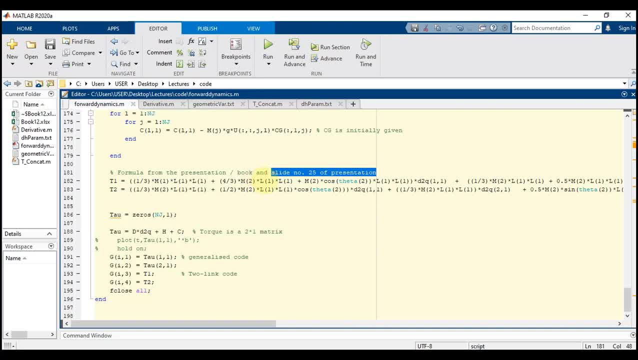 Which is similar to the expression in the book Foley and Gonzalez. This is the final expression of torque. Gi1 gives torque 1 from the generalized code. Gi2 gives torque 2, that is torque at joint 2, using the generalized code. Similarly, Gi3 and Gi4 gives the torque values for the two link code here. 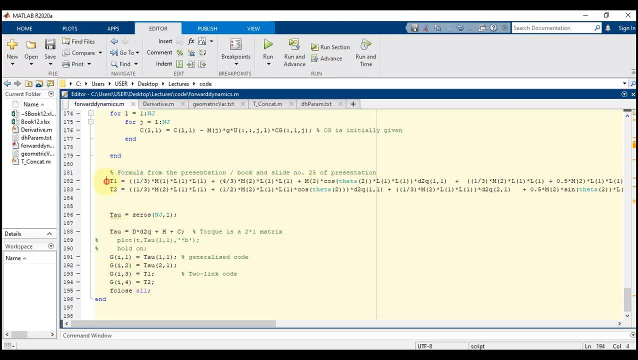 That is, Gi3 and Gi4 are nothing but this T1 and T2. Now let us verify whether Gi1 torque 1 and Gi3 torque 1 for the specific two link are matching And similarly, This torque 2 from here and this torque 2 from here have to match. 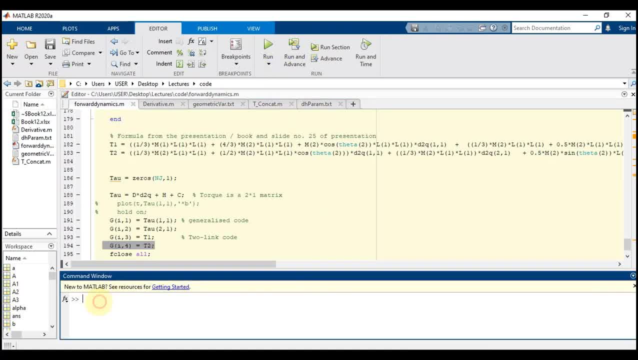 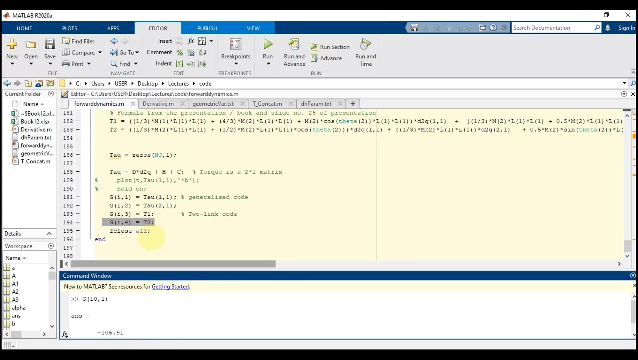 Let us run this code. For example, let us take G10,1. I can be anything Which is minus 106.91. Now this is torque 1 using the generalized code. Let us see what is torque 1 using this expression. So we have to: